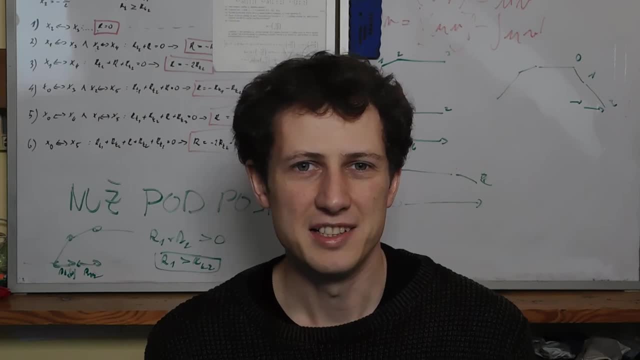 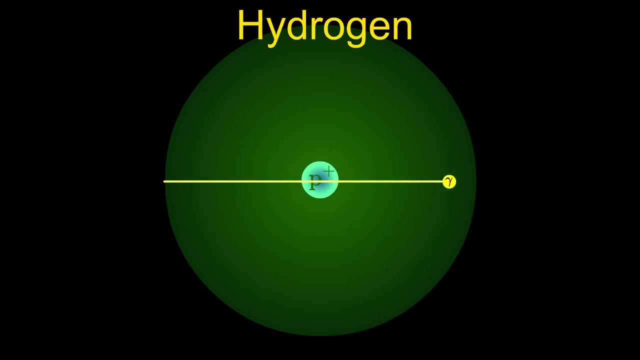 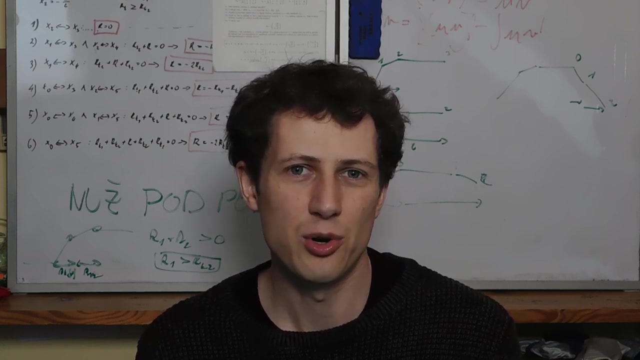 The smallest time period we have ever measured is 247 zeptoseconds, which is the time it takes for a photon to cross a hydrogen atom. But still the lifespan of, for example, Z boson is five orders of magnitude shorter. So how can we claim to have detected it In ideal world? 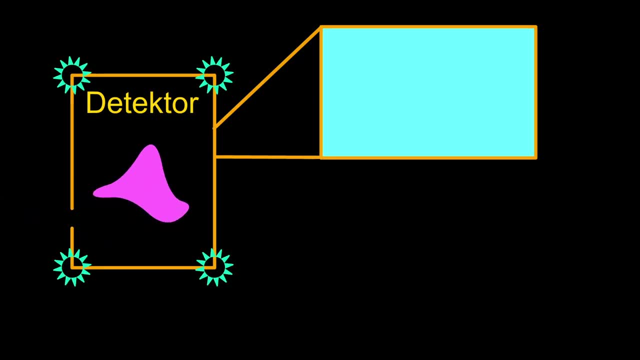 you would have this machine where you put matter in, then you run it and it will show all the particles that are in it. This is the time period we have ever measured. The smallest time period we have ever measured is 247 zeptoseconds, which is the time it takes for a photon to cross a hydrogen. atom. So how can we claim to have detected it? In ideal world, you would have this machine where you put matter in, then you run it and it will show all the particles that are in it. This is the time period we have ever measured. This is the time period we have ever measured The 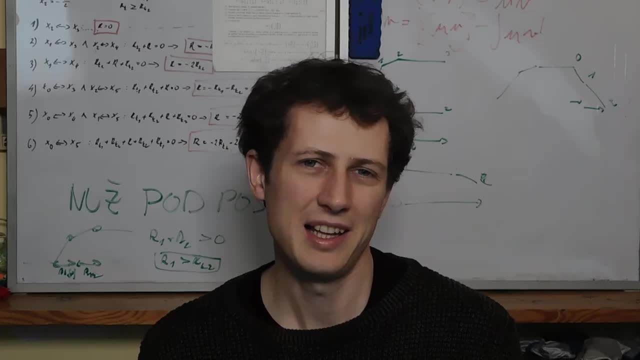 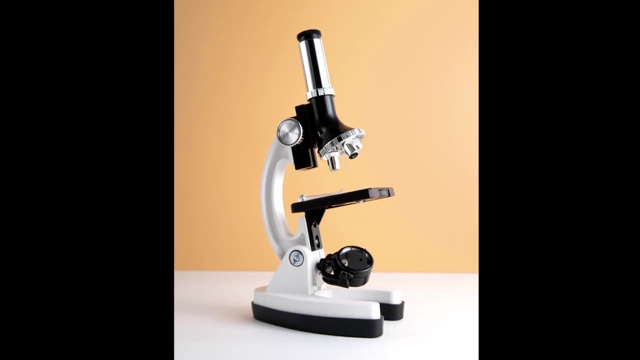 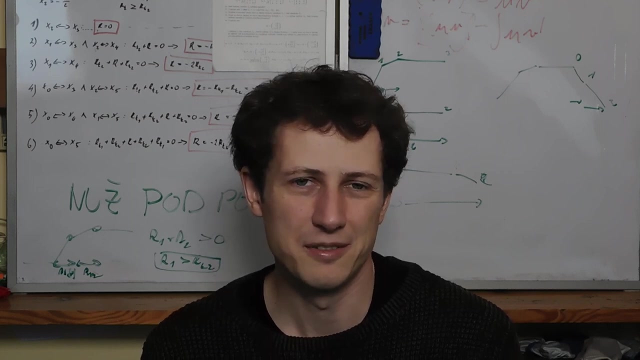 matter consists of on the display. In reality, though, building such machine is challenging, but we have some, For example the optical microscope. But no matter how advanced the microscope is, we are still limited by the wavelength of the visible light, So we can't. 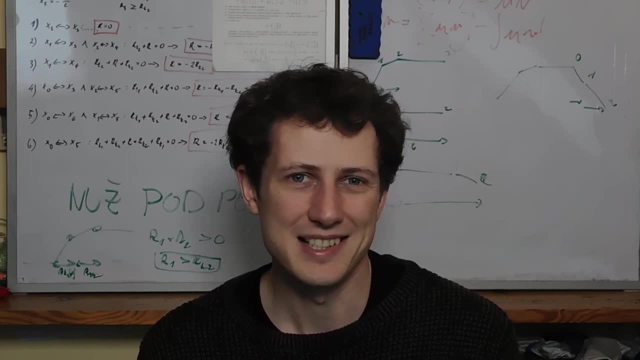 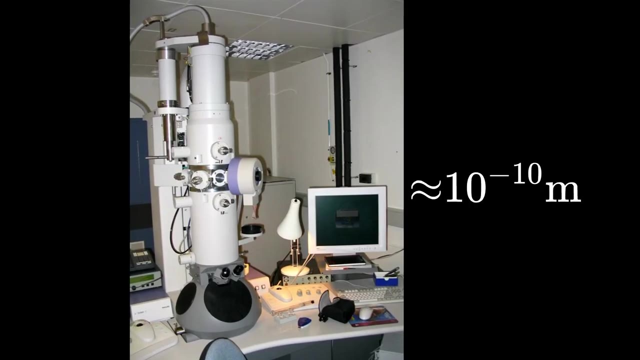 observe anything smaller than 10 to the minus 7 meters. If we don't limit ourselves to a visible light, we can use the electric field. This is the time period we have ever measured The electron microscope, which can get us much deeper into the matter. But how deep do we have to really? 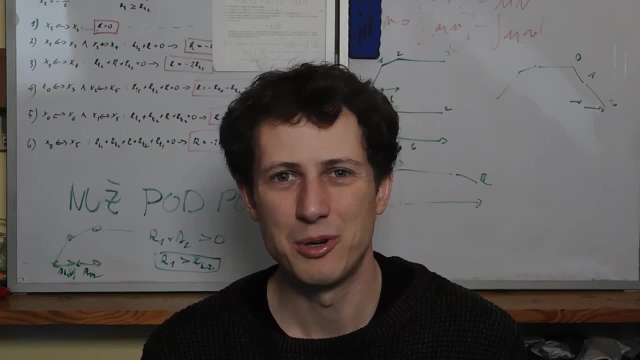 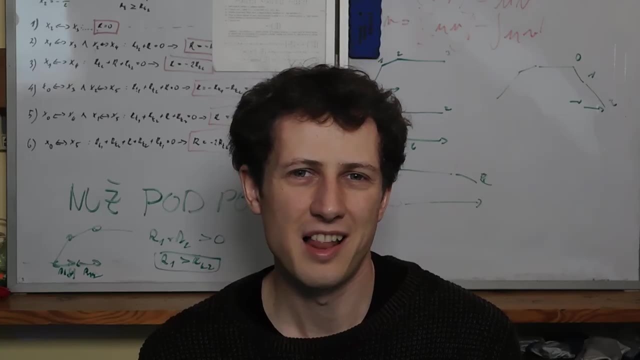 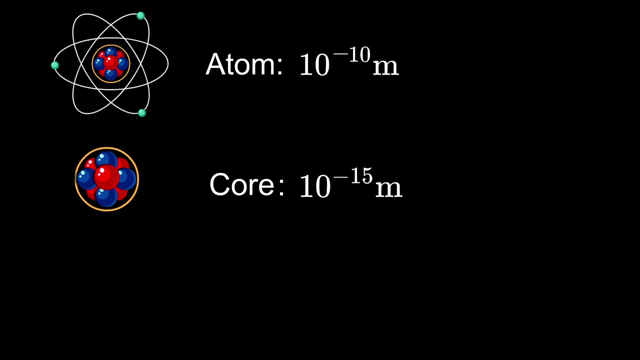 go to discover any particle. in the standard model, The typical size of atom is 10 to the minus 10 meters, which is still a very large object in particle physics. And if we talk about the atomic core, the size is much smaller, just about 10 to the minus 15 meters, which is 100,000. 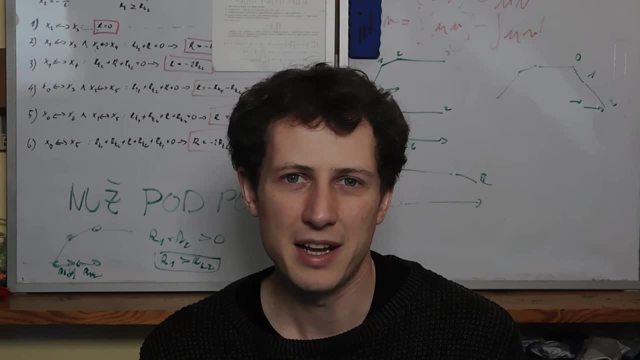 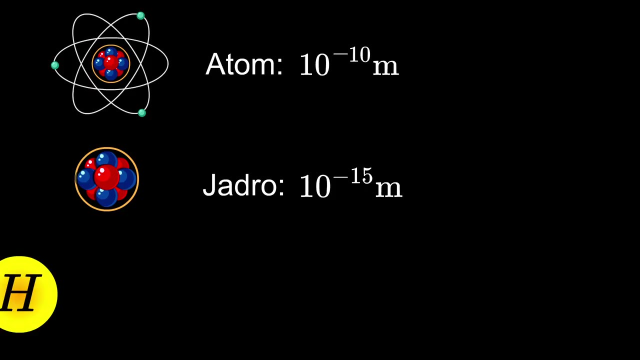 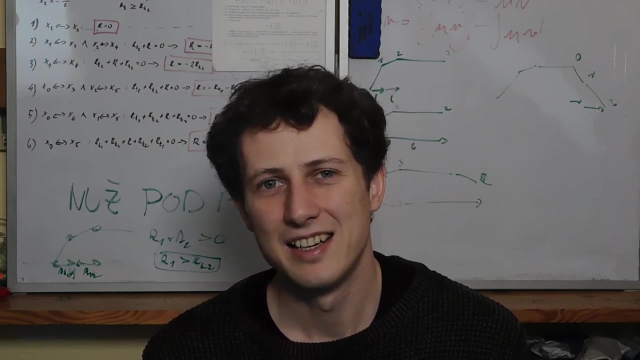 times smaller than the resolution of the electron microscope. And it is still not an elementary particle because it's made of quarks. So how big is actually an elementary particle? The problem here that, according to the current understanding, they don't have any size. 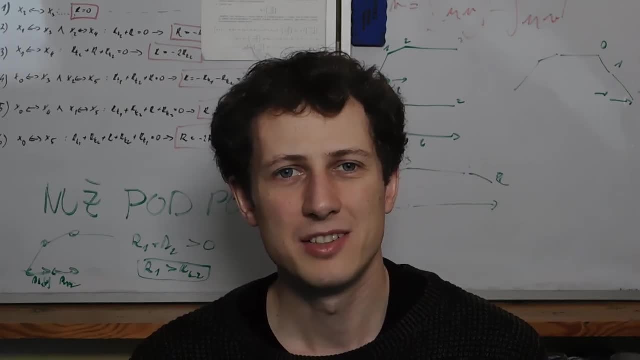 So how can they be detected? Well, at this point there is not much we can do in terms of direct detection And we have to use indirect methods, especially if we want to be able to detect anything. So we have to use indirect methods, especially. 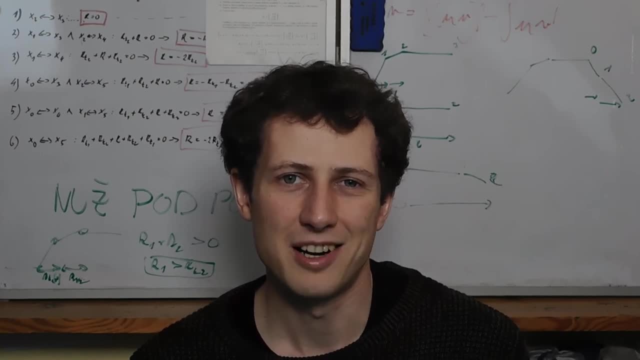 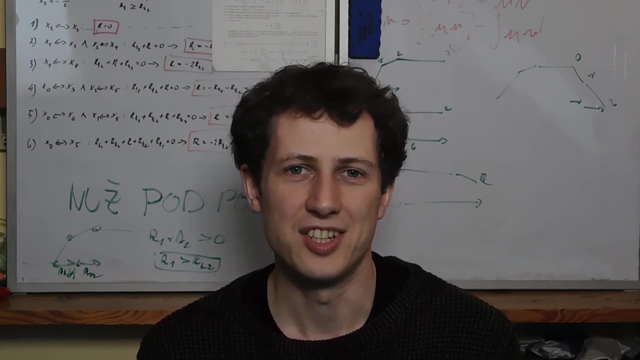 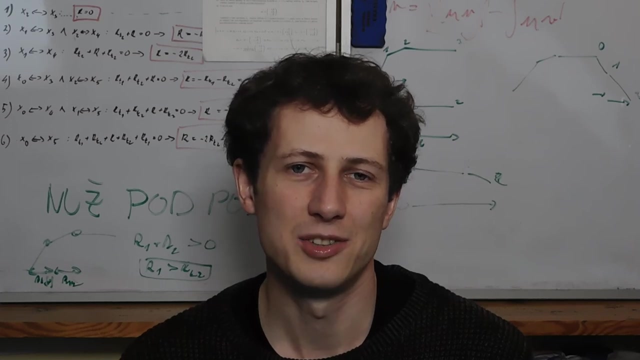 if we study the influence of the particle on the surrounding matter, When a charged particle is moving through a medium, there is a lot of ways it can lose its energy, like collisions, excitations or Bremsstrahlung radiation. The details of these are not important for us, but 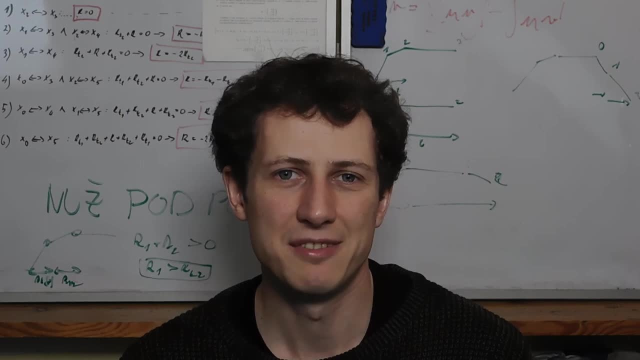 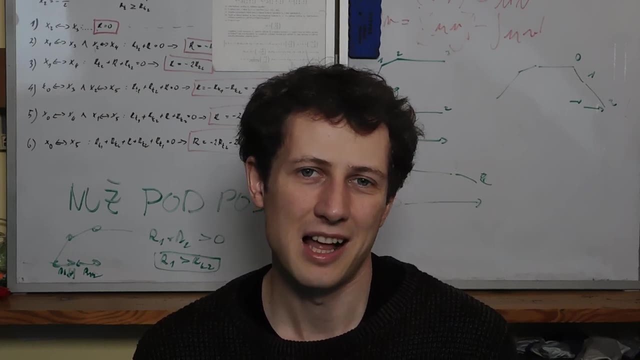 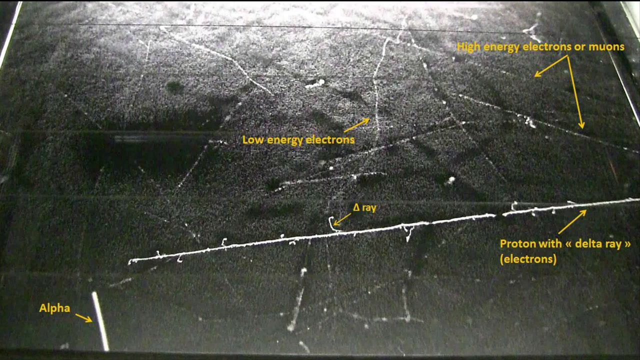 what is important is that different particles have different influence on the surrounding matter. One of such detectors is the famous cloud chamber, As you can see on the picture here, we have different ionizations for different particles like alpha particles, protons or electrons. There is also a difference between 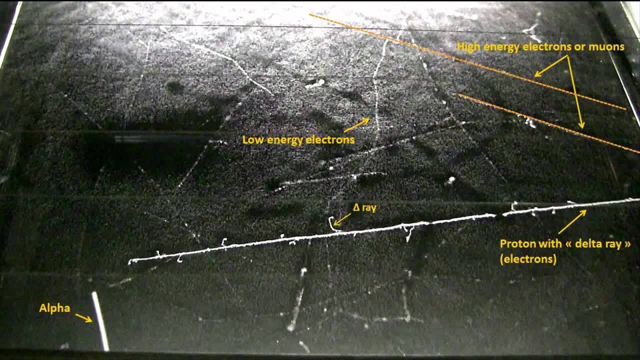 electrons of different energy, as you can see here, where electrons of high energy travel in a straight line, whereas electrons of low energy are kind of wandering in the medium. Moreover, if the particles are moving in a straight line, then the electrons of low energy are kind of wandering in the medium. 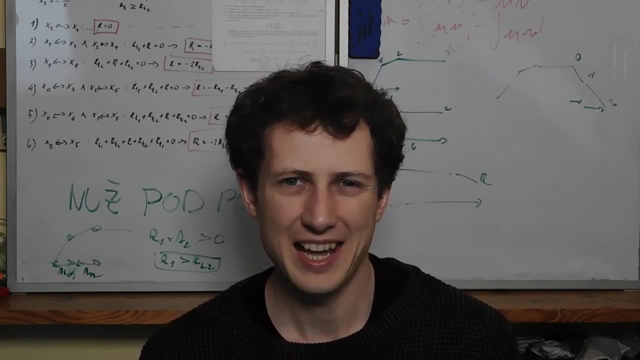 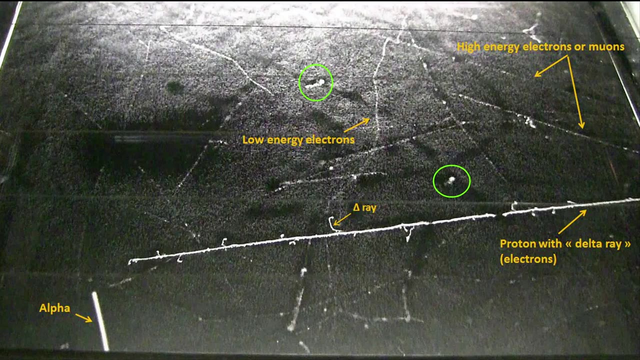 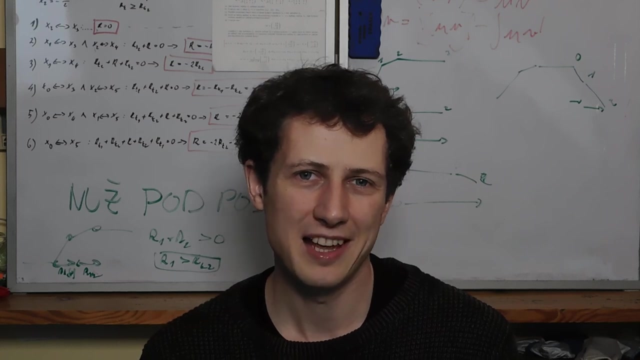 If the particle is not charged like photon, we don't see any track in the cloud chamber. But what we see are these dots, which are the spots where the photon hit something, creating a local ionization. You can also add a magnetic field and then you are able to detect the sign of a 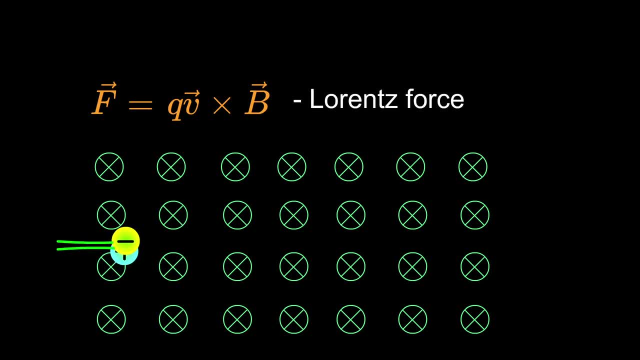 charge of the particle. As the particles with opposite charge curve differently in magnetic field, creating different tracks, then you can not only detect the charge of the particle, but also can not only detect the charge of the particle, but it also tells you something about its momentum. 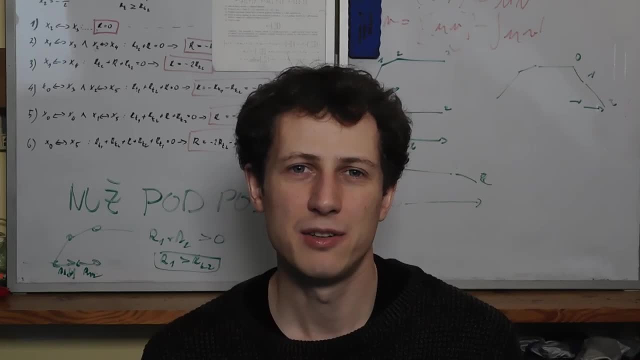 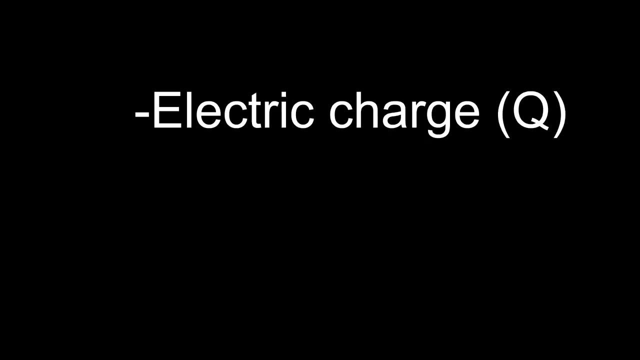 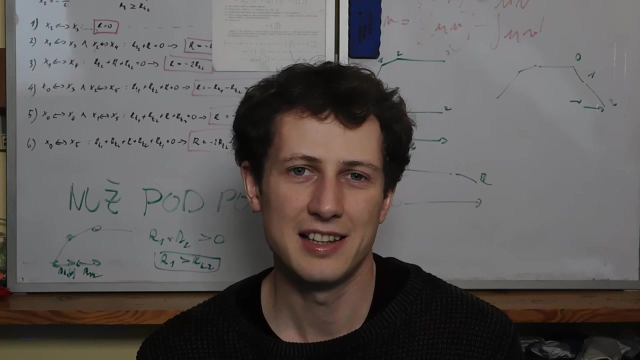 depending on the track radius. The bottom line of all this is that we can create detectors that can measure the electric charge of the particle and the momentum of the particle. This is still not enough, because we need to know whether the particle we have detected was truly elementary. 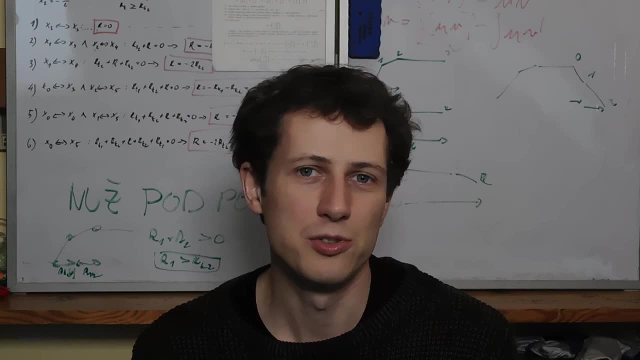 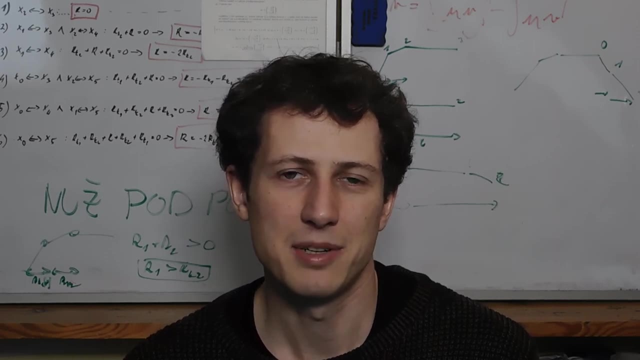 and not some kind of hadron-like product. If the particle we are detecting is some kind of lepton, then we know that it interacts predominantly via electromagnetic interaction, And there is a special type of detector meant to capture all the energy of such particles. However, this requires the particle to not be very massive. 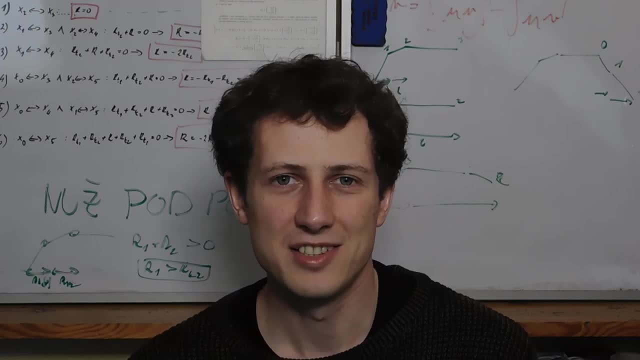 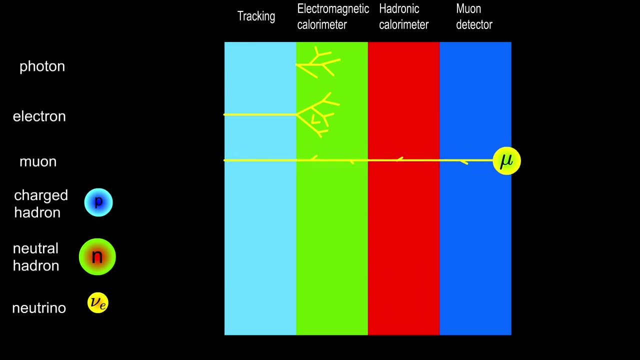 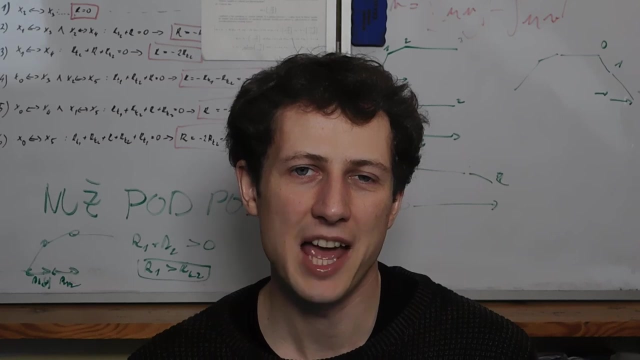 because otherwise the electromagnetic interaction is not strong enough to stop the particle. This is the case for muon, which is a lepton 200 times heavier than electron, which can easily penetrate this calorimeter. But this is also a good thing, because heavier hadrons. 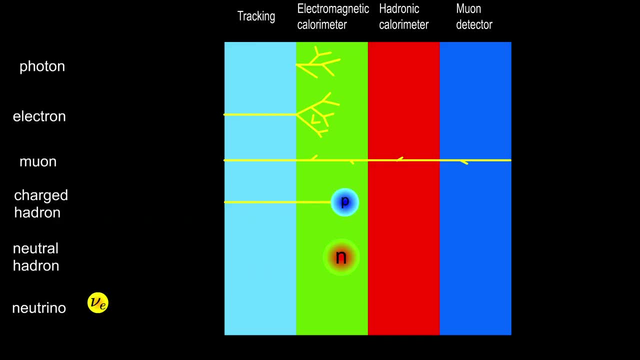 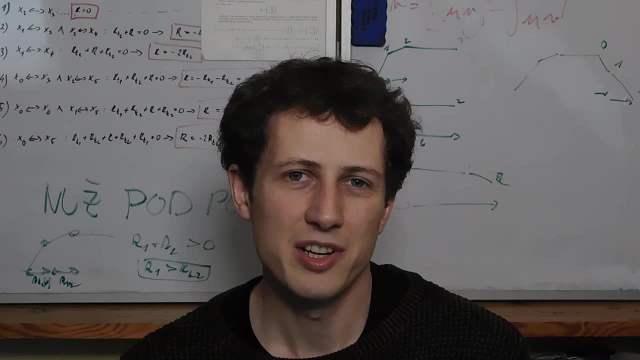 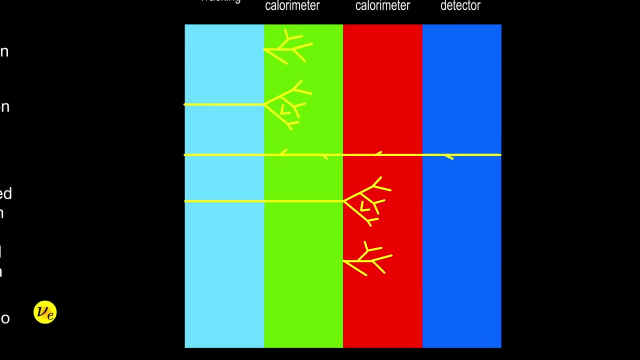 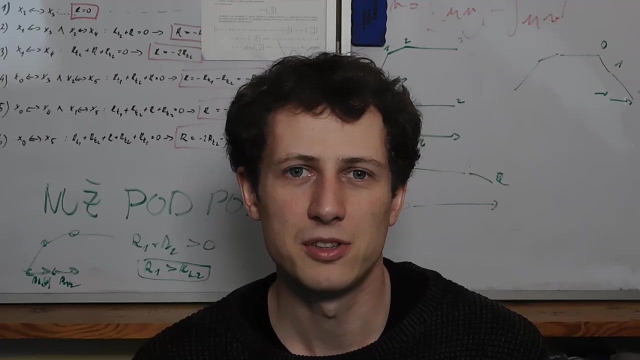 like protons or neutrons, can also easily penetrate this calorimeter. But apart from muon, these particles interact predominantly via a strong interaction, and this is the reason why we use different type of calorimeter to measure the energy of the particle. So now we can distinguish electrons and photons from hadrons and since the problematic muon does. 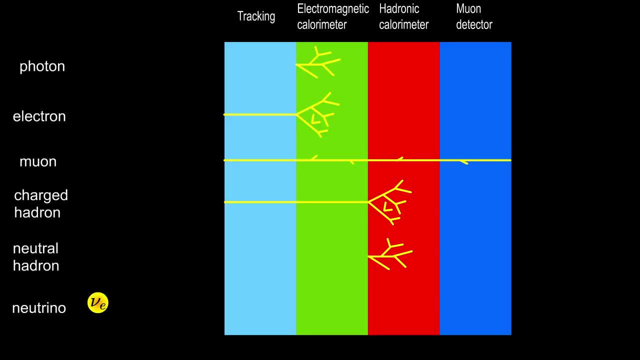 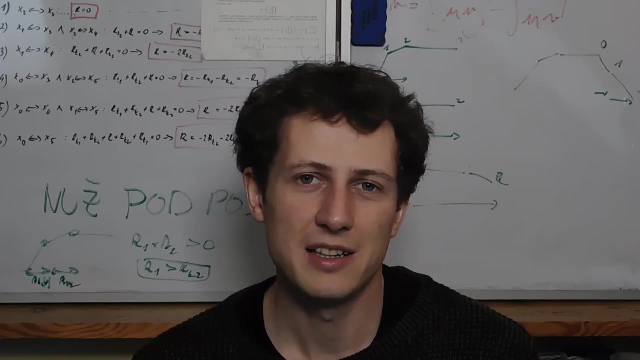 not interact strongly, it can easily penetrate hadronic calorimeter. So there is another layer called muon chambers, where if we detect something coming from the detector, we know it's muon. So detection of muons is in fact very easy, even though it's really hard to capture them in the detector. 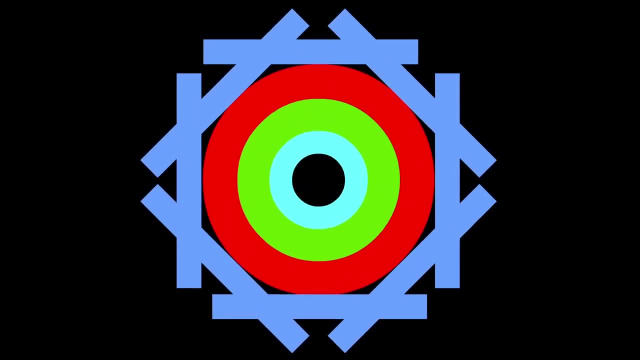 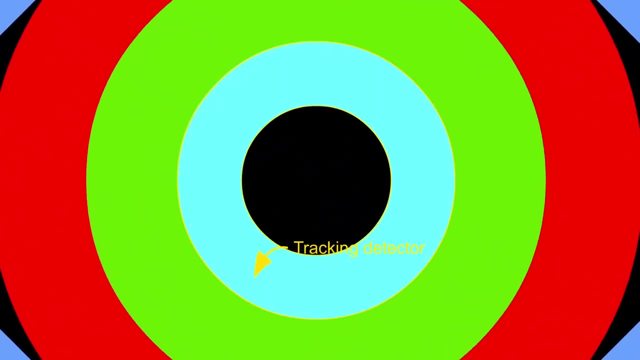 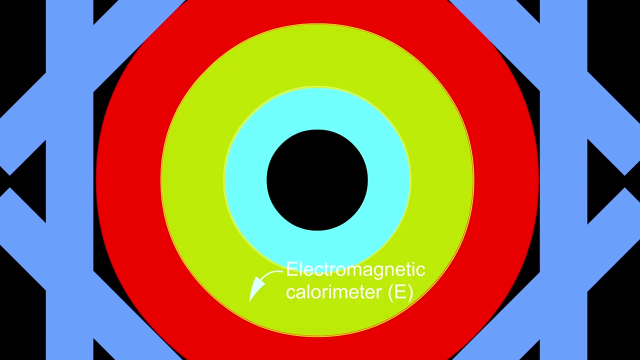 To summarize, we can create a schematic version of the ATLAS detector at LHC, where this inner layer is track detector, meant to measure the charge and momentum of the particle. Next is electromagnetic calorimeter, meant to capture all the energy, photons and electrons, which is particularly 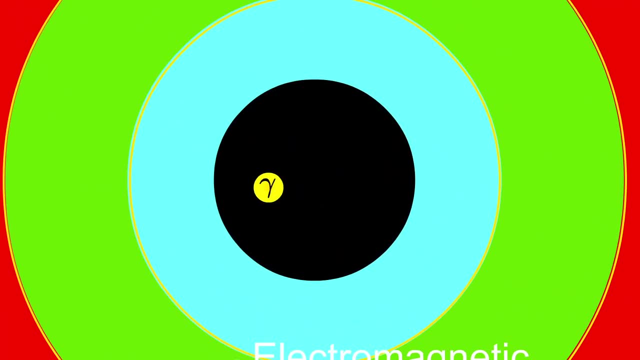 important for photon detection. So this layer is a track detector meant to measure the charge and momentum of photons because since they are not charged, it won't leave a track in tracking detector And therefore we can only measure its energy and therefore momentum here. 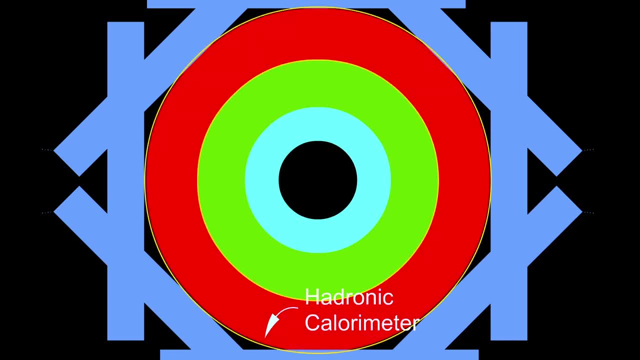 Next is hadronic calorimeter, meant to capture all the energy of hadrons, but you can immediately forget about this part, because detecting particles using hadronic calorimeter is difficult and most new particles were detected through leptons. The final part of the detector is the energy of the particles, which is the energy of the particles. 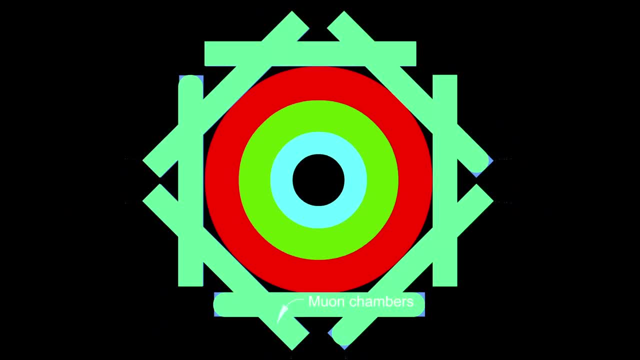 The final part of the detector are muon chambers meant to detect the strongly penetrating muons, And this is what we are going to see on the detector for each particle. For photon, we only see the energy deposition on the electromagnetic calorimeter and nothing else. 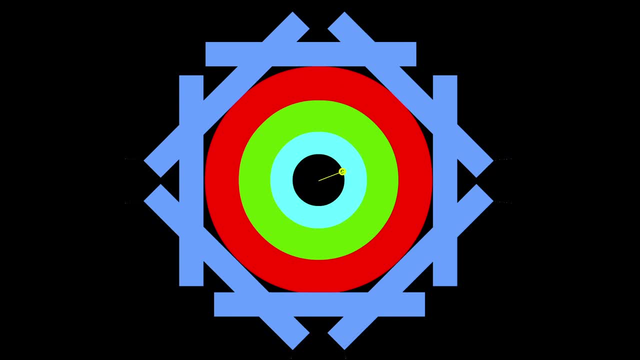 since it's uncharged, Electron leaves the track in the tracking detector and deposits all its energy in the muon chambers. Muon is going to leave a track in the tracking detector and penetrates the entire detector, leaving a part of its energy everywhere, also in the muon chambers. 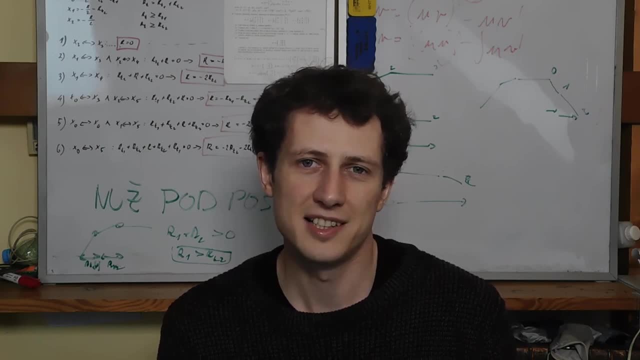 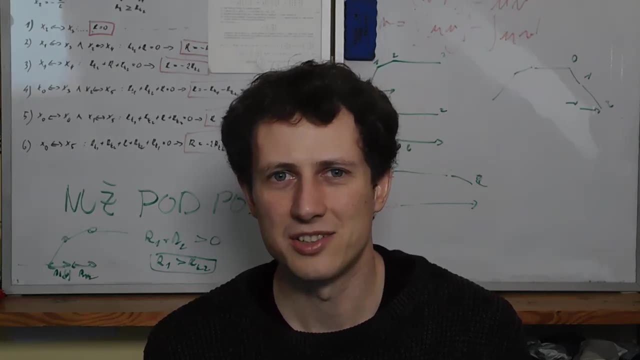 And these are all the particles we are interested in, since we don't want to deal with hadrons. Okay, I know what you're probably thinking of. We can detect photons, electrons or even muons, but those are stable particles. But what about these weirdos with? 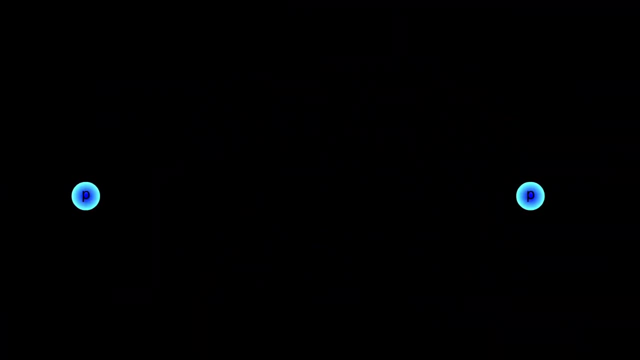 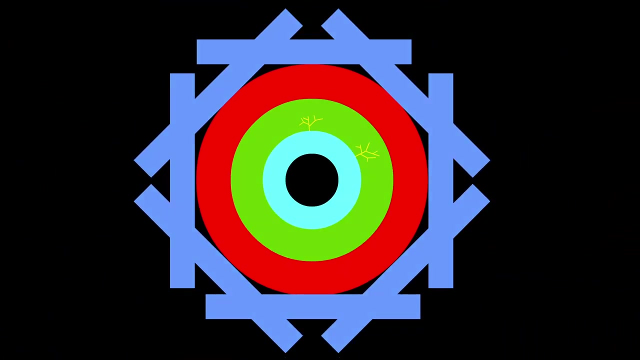 such a short lifespan. If we collide two protons and create a Higgs boson, then it immediately decay and even if it traveled with the speed of light, it would cover just a distance as short as the diameter of a proton. And what we truly detect are the final decay products. 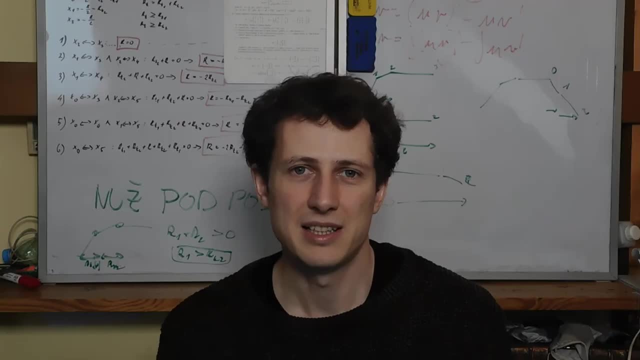 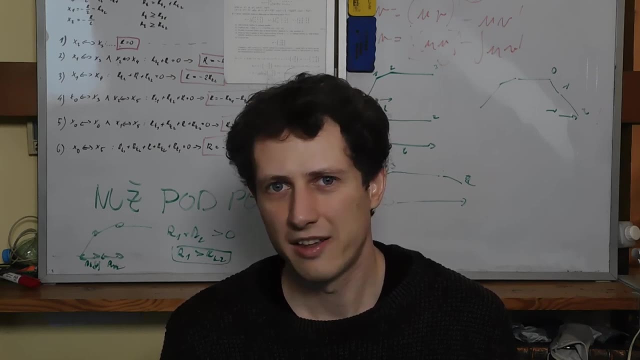 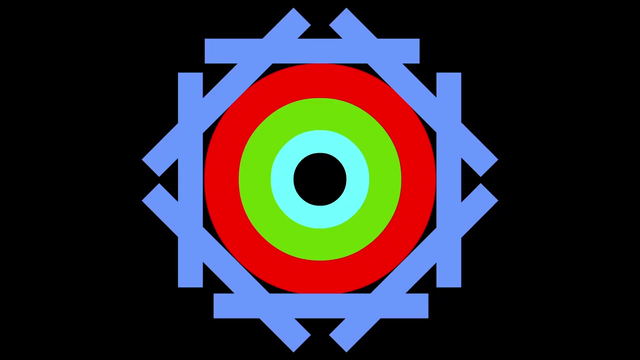 which in this case are two photons. But since I teach special relativity, you probably already know that there are phenomena like time dilation or length contraction, depending on which reference frame you choose, For example, from the frame of the Higgs boson. 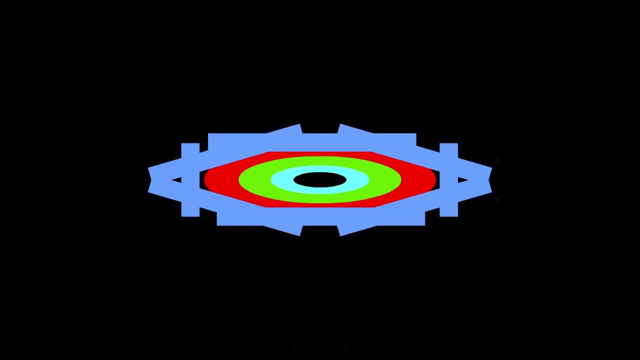 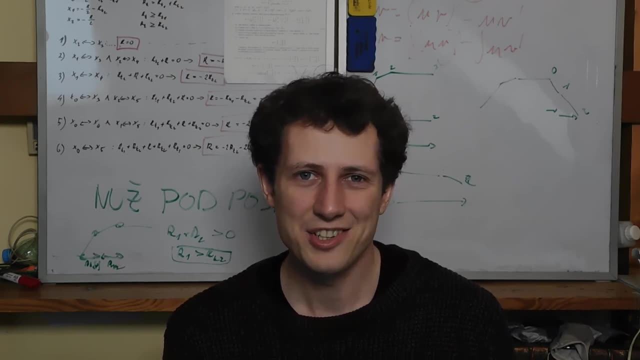 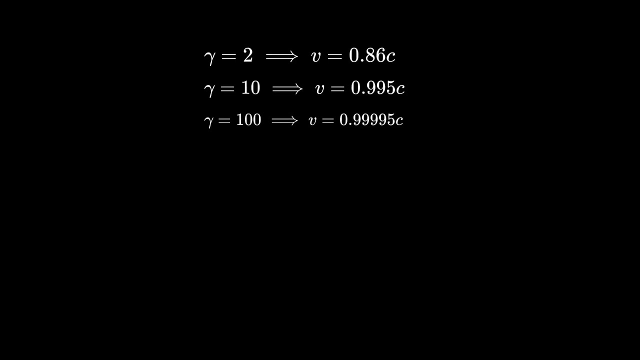 the detector looks more like this, where it shrinks in the direction of motion, But could the length contraction be so extreme that the Higgs boson could eventually hit the detector? The amount by which the length is contracted is represented by this gamma factor, which tells you how many times is the length shorter relative to the detector's. 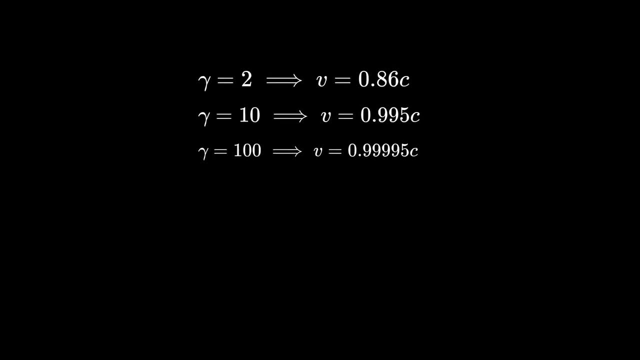 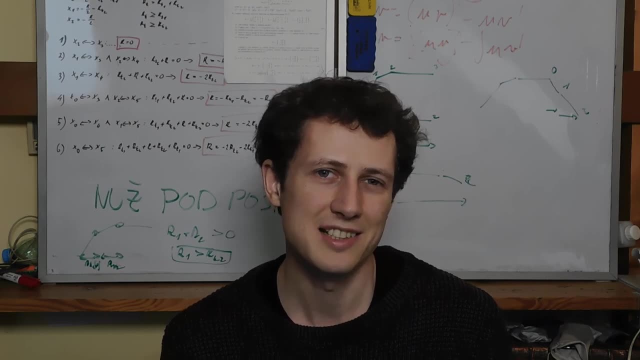 rest frame for any given velocity of the Higgs boson And i calculated how fast would have the Higgs boson go in order to cover the distances in the order of one meter and i got this crazy number. You can also calculate its energy it would have. 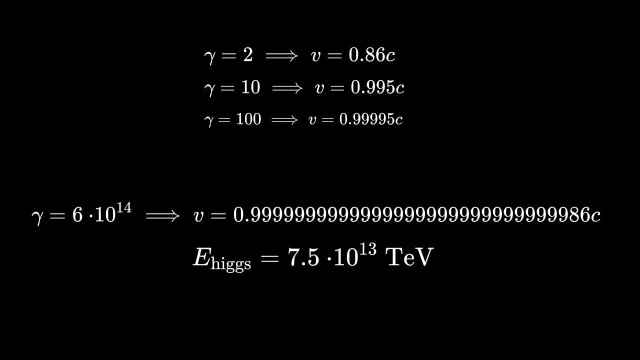 to have for this velocity, and I got the number in order of 10 to the 13 tera electron Volts, But the energy at which LHC operates is just 3 times less. excuse me, you can also calculate its energy. it would have to have for this velocity, and I got the number in order of 10 to the 13 tera electron volts, but the energy at which LHC operates is just 3 times. 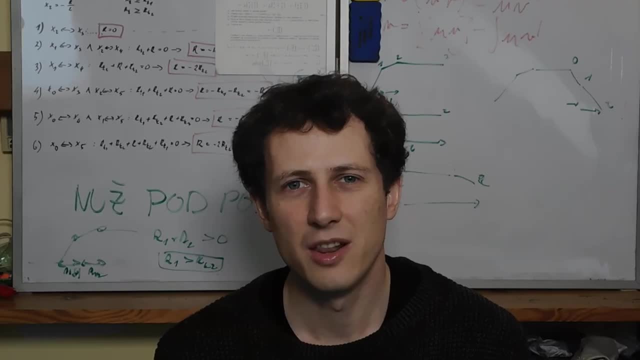 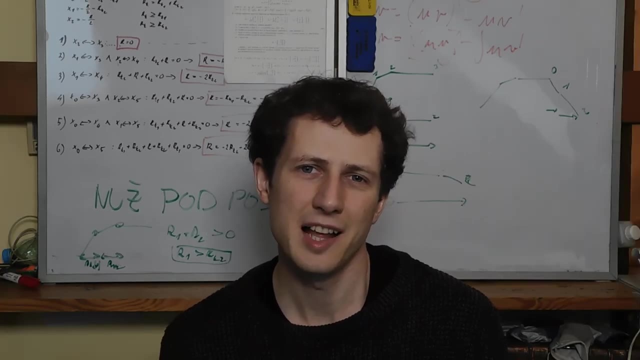 You can calculate the third energy, which takes 4 seconds. Well, and when you see the general radius of the detector: 13 teraelectron volts, which is significantly lower. and there is just no way we can create Higgs boson with this energy ever. But physicists still claim to have detected it. But how? Because 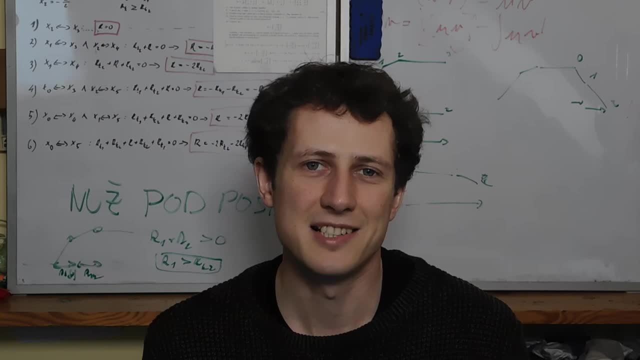 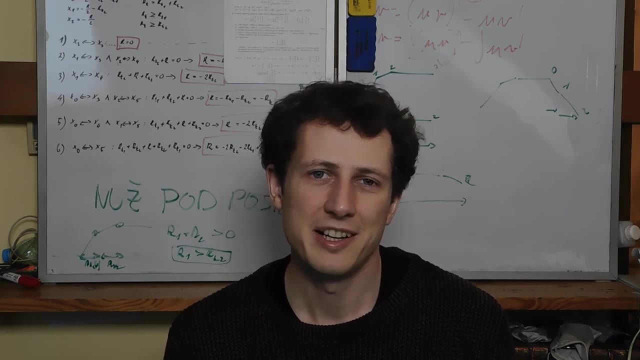 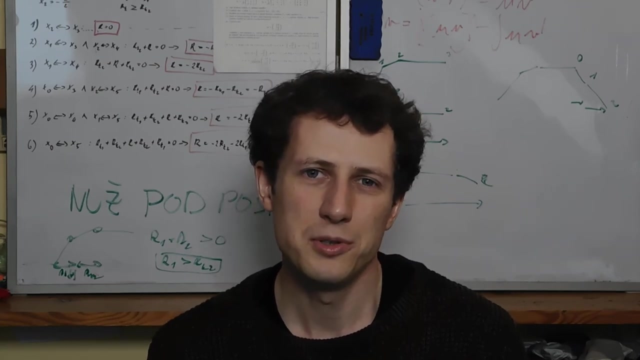 there are many ways how to create two photons in a final state, So how can we know they come from Higgs boson? To understand this, we need to talk about the invariant mass, which is extremely useful quantity in particle physics. The reason why it's so useful is in the name: invariant. 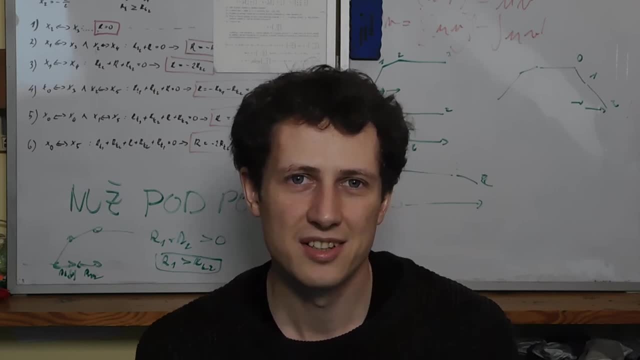 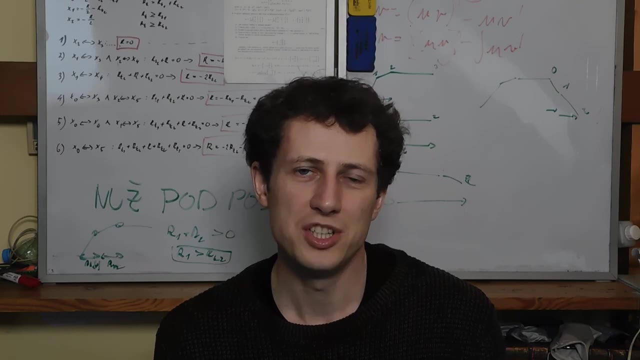 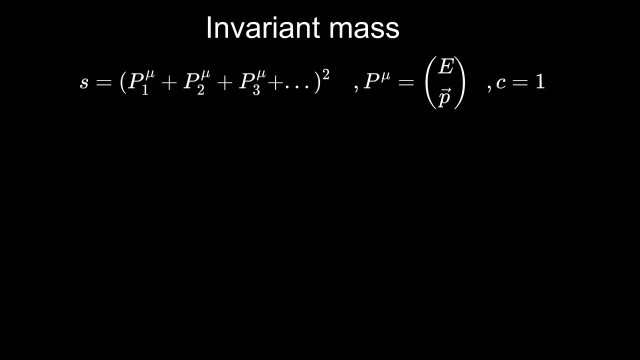 which means that this quantity doesn't change. It doesn't change when you change your frame of reference, but it also doesn't change before and after collision or decoy. The definition of this quantity is just simply squared sum of the particles for momenta, If you have just a single. 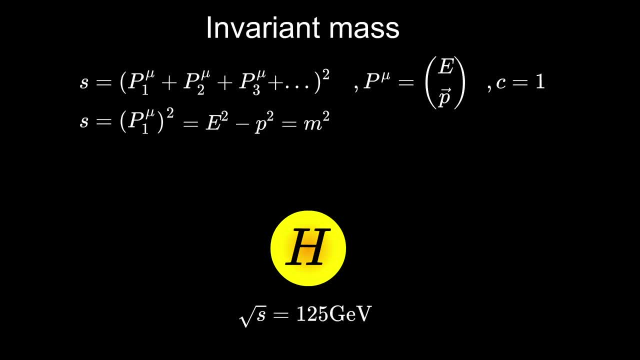 particle, then it's invariant. The invariant mass is just its own rest mass. This is also true even if the particle is moving relative to us, because the total energy and momentum exactly compensate to the same number of 125 GeV. If the particle decays into two other particles, then based on their energy's momentum, 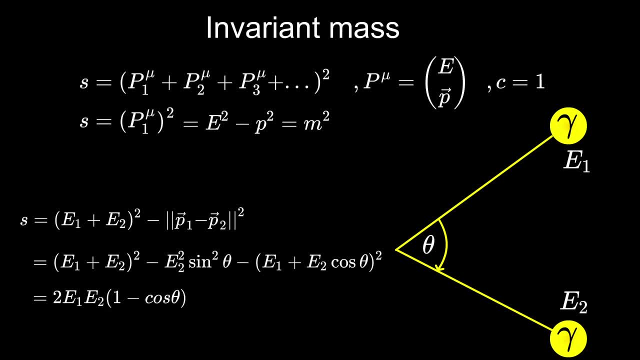 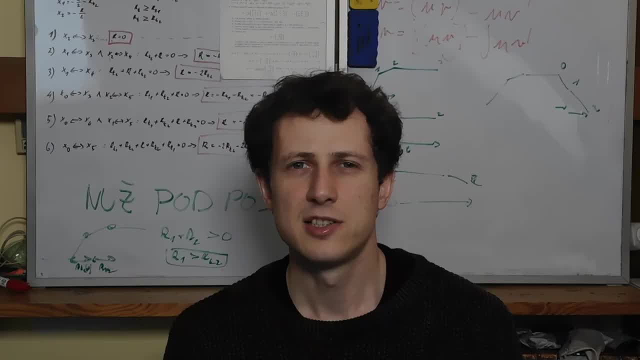 and the angle between them, you can calculate the invariant mass of these two particle systems And in the case of Higgs boson you would get 125 GeV. So let's consider this decoy channel of Higgs to two photons, Even though 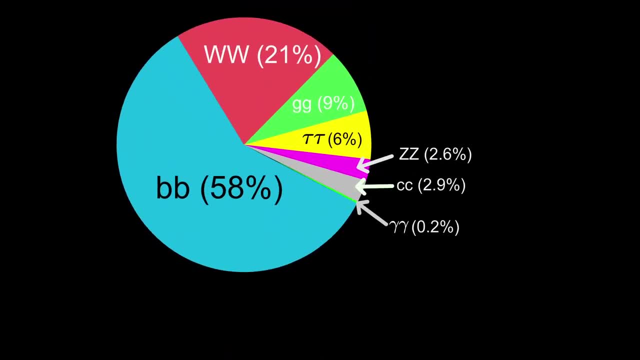 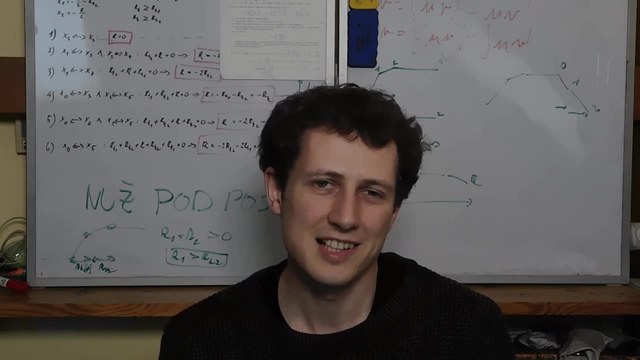 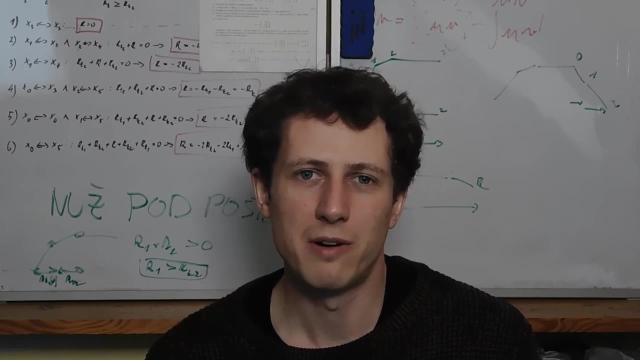 the probability the Higgs decoying into two photons is just 0.2%. photons are so easy to detect that it was in fact this channel that led to the discovery of the Higgs boson in 2012.. The discovery of Higgs decoying into two bottom quarks happened after five years, even though it's the dominant 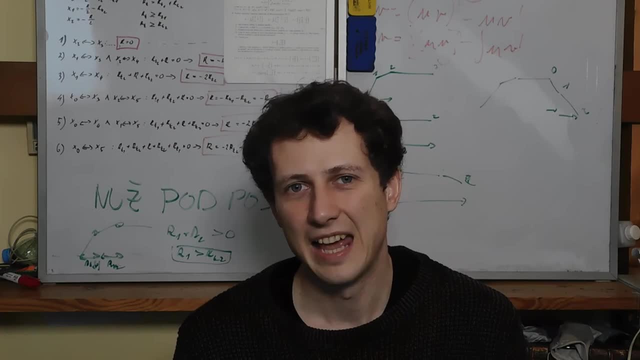 decoying channel. So let's consider this decoy channel of Higgs to two photons, Even though the probability the Higgs decoying into two photons is just 0.2%. photons are so easy to detect that it's Higgs. des Yoshino, Hildebrandt, Hadrons are hard, as I said. Anyway, now if we detect 2 photons in the 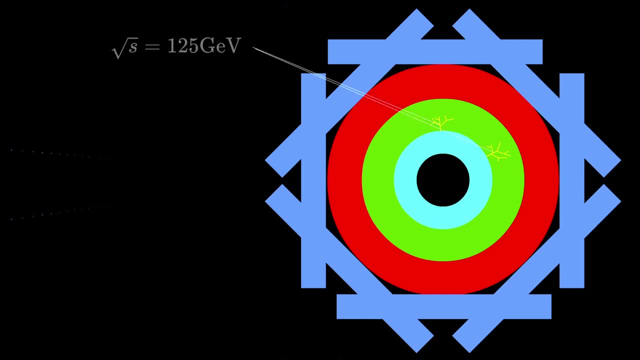 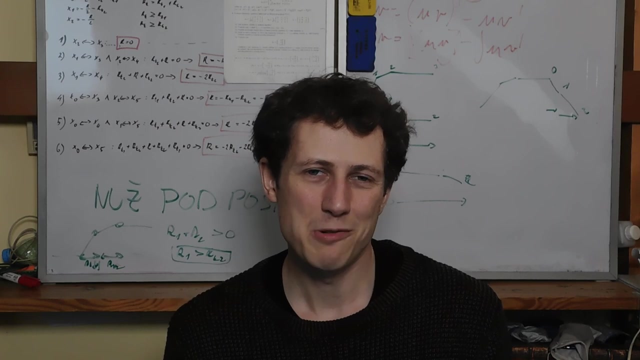 detector… and since we can measure their energy, we can calculate the invariant mass And if we get the number of 125 GeV, we have the Higgs right. I must disappoint you, guys, but I wish it was that simple. But we need to go back to coast, to reality. All we can say is that it is a candidate. for Higgs. I hate Higgs because of their numbers and their hardness, but this is just way too straightforward. Higgs is broken here. UnmStationable bushings and no net-pочhabitude hit auch an infinite number of levels. 그� diferre vuh-zu. 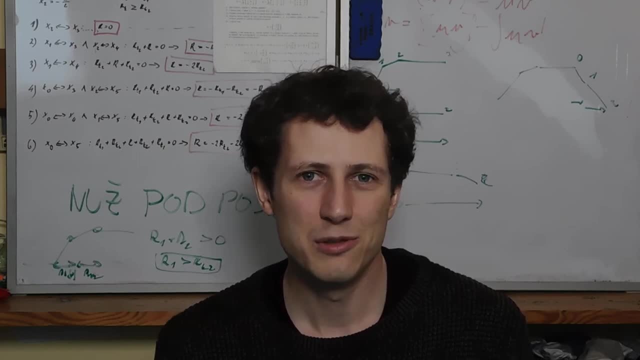 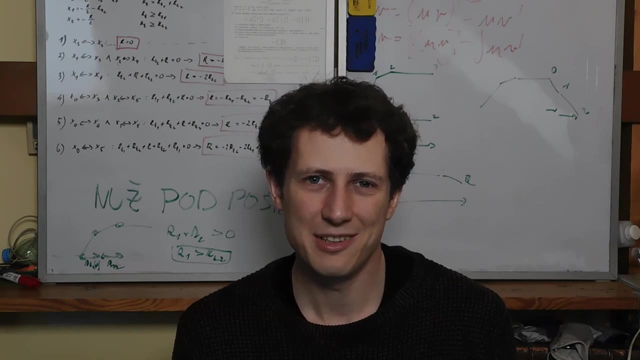 again, there are many ways that can decoy into two photons with this particular invariant mass. But isn't it weird? I said that the invariant mass is conserved and if we detect two photons with the invariant mass of 125 GeV, it must have been created from something that have the same. 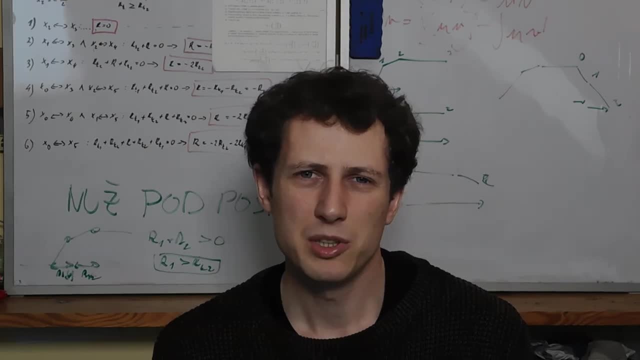 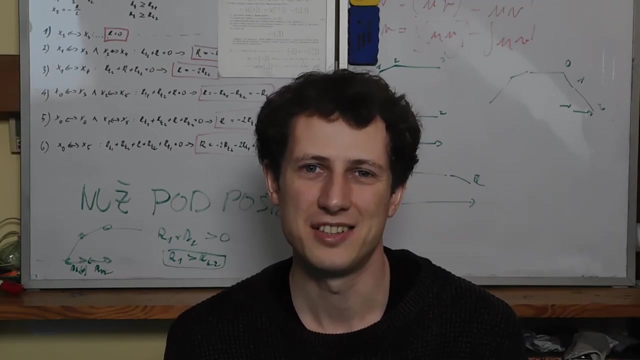 invariant mass in its rest frame. right, But what other particles have the same mass as the Higgs boson? that would produce two photons in the final state with the invariant mass of 125 GeV. And the answer is even worse than you can imagine, because it is in fact every single particle in the universe. 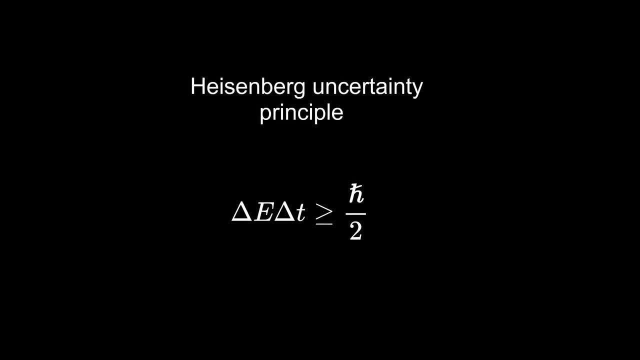 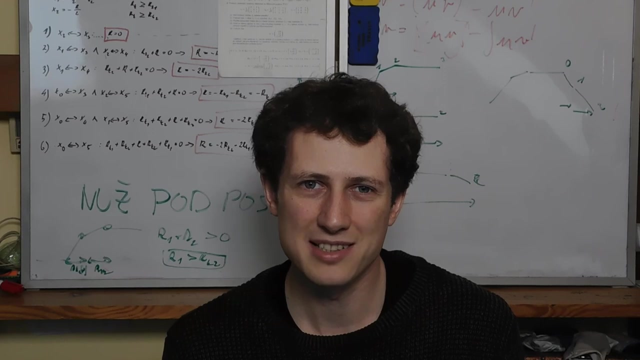 Do you recall the Heisenberg uncertainty relation? If you just switch energy for mass, you find out that the mass of the particle is uncertain and the amount of uncertainty depends on its lifespan. So any particle can be created with any mass, as long as the Heisenberg uncertainty principle is satisfied. 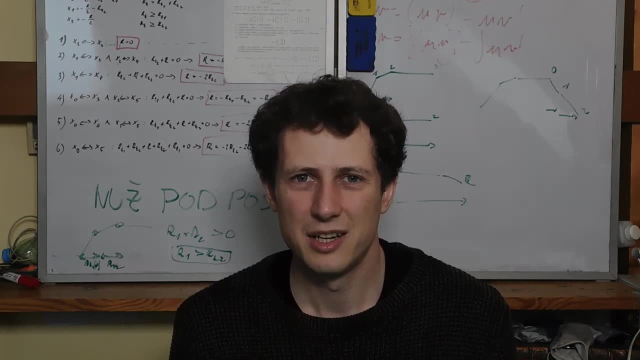 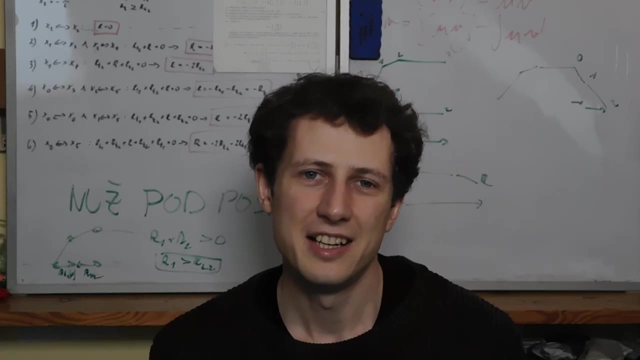 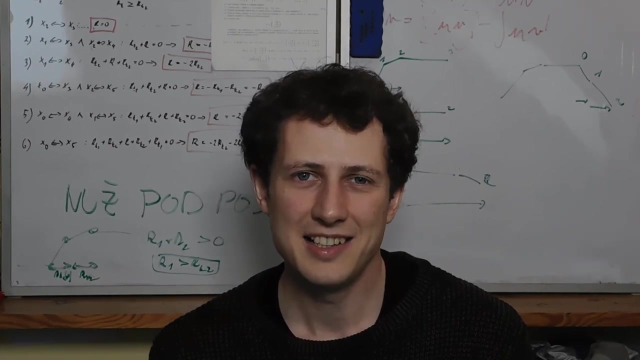 So it feels like we are losing ammunition here. What else there is left for us to do if we can't even know the masses exactly? Fortunately, there is one trick we can use. The trick worth of dozens Nobel prices, and it is the fact that particles like being created with their real mass, If you. 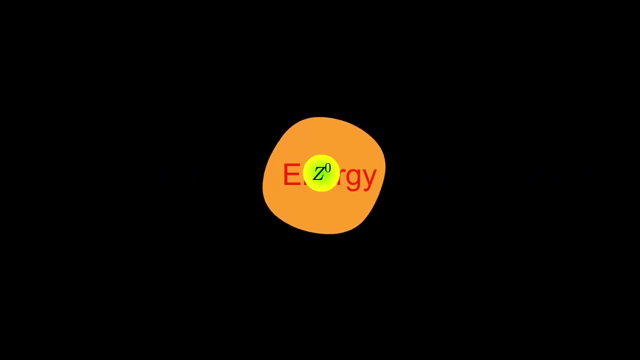 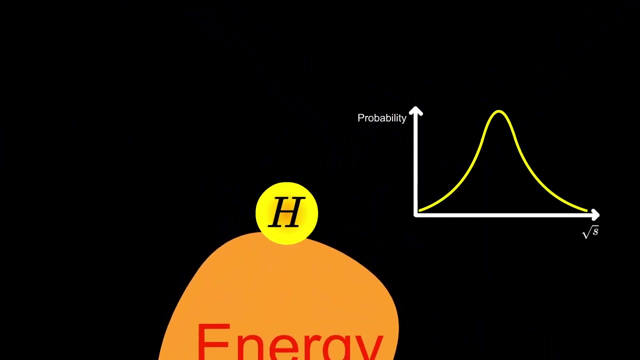 divide that two protons, you get this energy soup where particles are created. If the Higgs boson is created, the most likely it is going to happen here, which is called the on-shell creation. The further away from its real mass, the less likely such creation is. This is the direct consequence of the 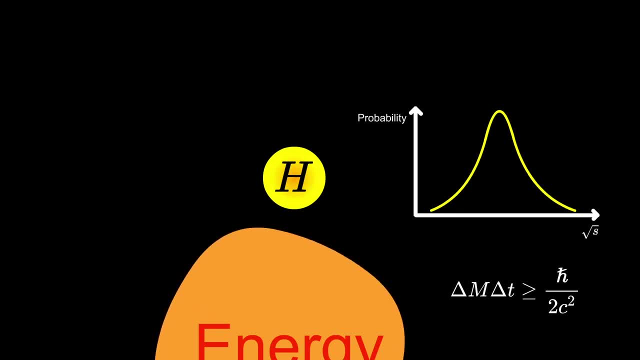 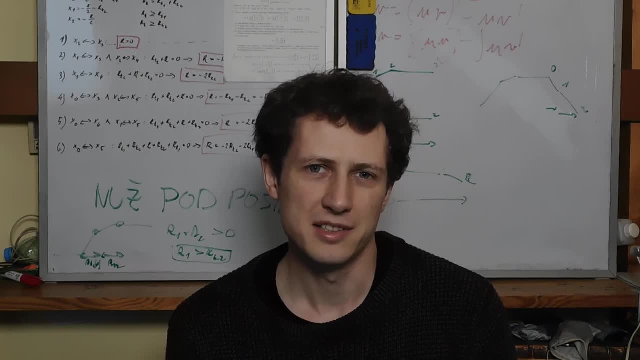 Heisenberg uncertainty relation, because the more stable particle, the narrower the peak is. So we can't know whether these two final state particles came from Higgs or some other particles, but there is this anomaly in the probability of creation, So we can use statistics now Instead of just analyzing. 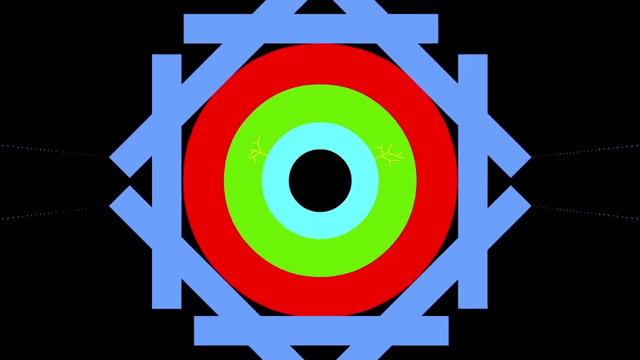 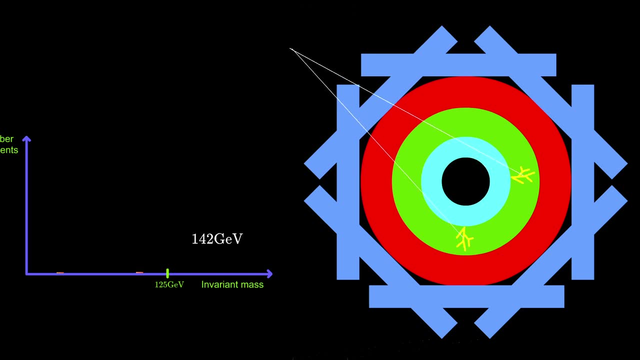 a single event of Higgs decoding the two gammas, we can analyze many. We calculate the invariant mass of each and form a graph of number of events versus the invariant mass of the photon pairs. And since there is a higher probability of creation at 125 GeV, it will eventually appear in 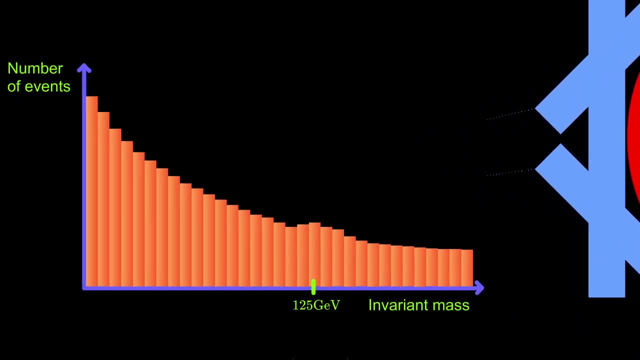 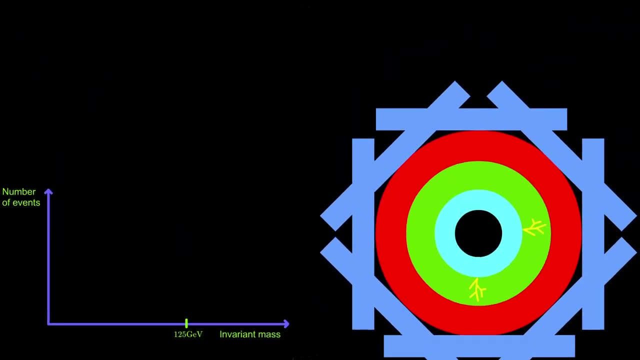 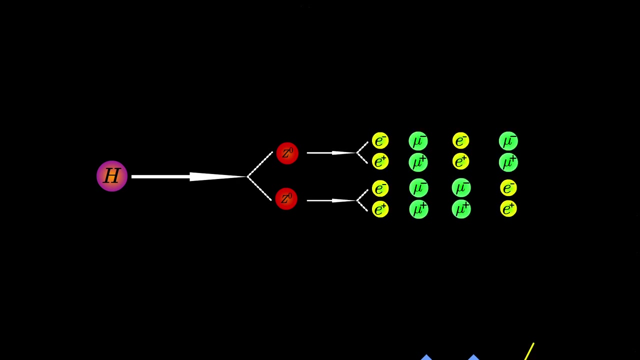 the statistics as a peak in the number of events with the invariant mass of 125 GeV. And you don't have to limit yourself to just two photons, because Higgs can also decoy into two Z bosons, which further decoy into leptons, and you can analyze the four lepton events and make the invariant mass. 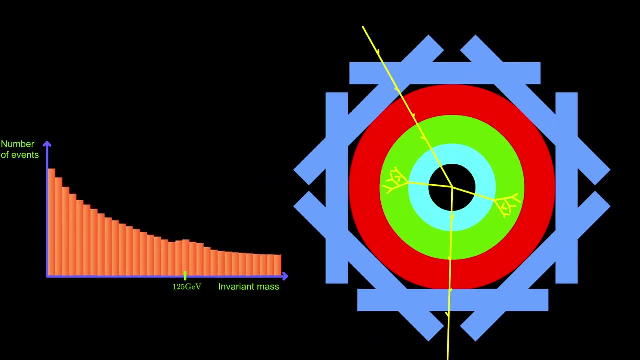 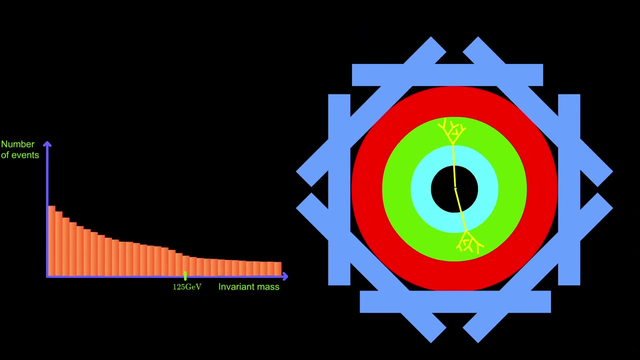 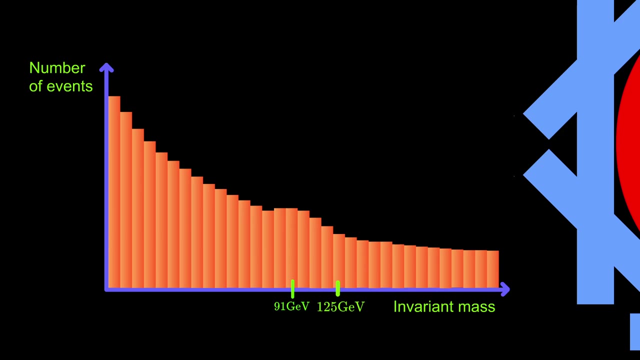 for this four lepton final state and you would see the same peak. Or if you analyze just two lepton decay, you would see the peak at 91 GeV and not 125 GeV because the probability of Higgs decoying into electrons or muons is basically non-existent, But for Z boson it is significant. 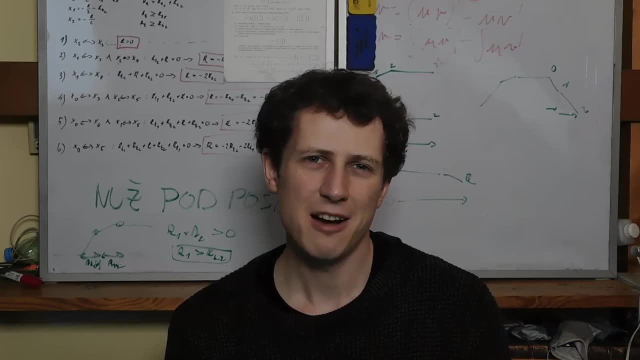 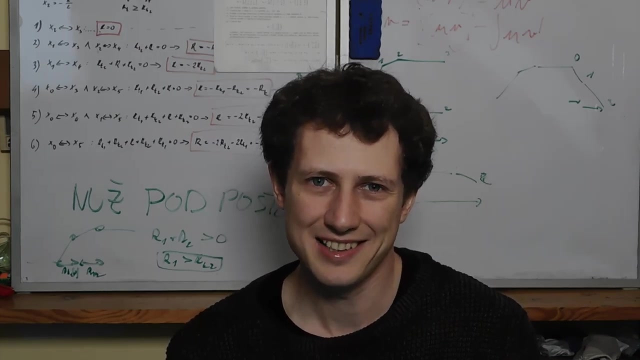 and this would be the discovery of the Z boson. And this is how physicists detect particles. They never observed one, they never isolated one, and they can never take a single event and say that there was a Higgs. Its presence appears only in the statistical data And, moreover, physicists can't. 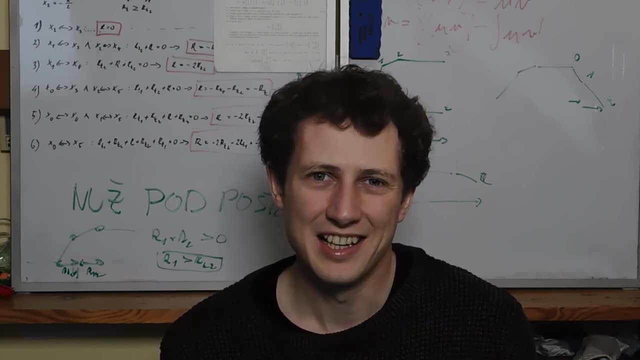 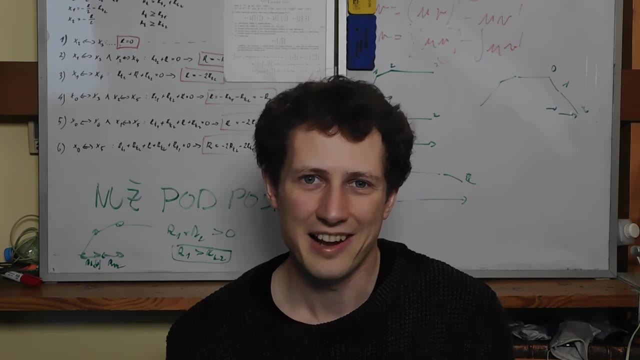 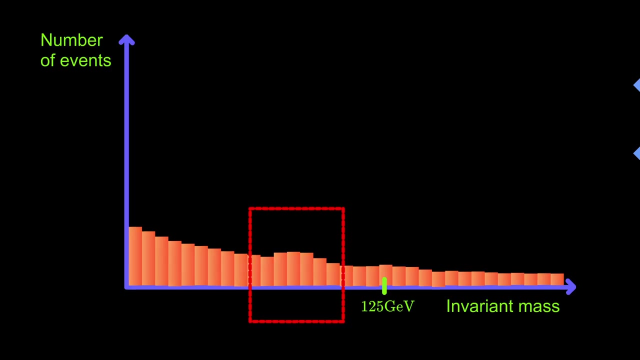 even say with 100% certainty that these particles exist or not. All they can say is the confidence level for their existence, Because when you do the statistics, there can be random fluctuations anywhere in the data that level up with more and more data, and we can never be.